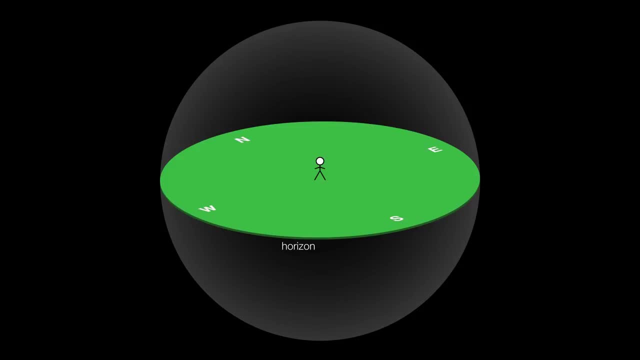 if you like. The horizon is just a perfect 360 degree circle and the sky is suspended both above and below us, And the reason why I've drawn it below as well is because we know from our experience that there are stars and planets that have yet to rise. They'll rise later this afternoon, and 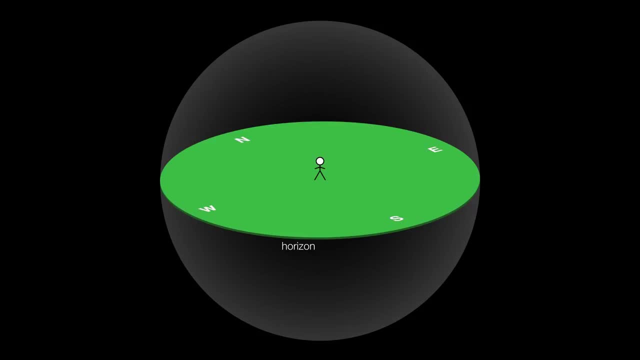 this evening. So we're going to go ahead and just represent the entire sky, even though we can't see it all. Now, the position that's directly above our heads is called the zenith, and the point directly beneath our feet we call that the nadir, And if we take a circle and draw it from due north through, 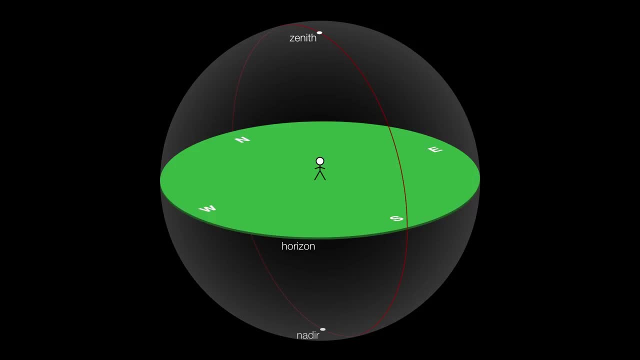 the zenith to due south and back around again. then we can define a circle that will divide the sky into eastern and western halves. This is called the meridian, and this is going to be a useful reference point going forward. Now, while we're here, I'd like to just describe for you briefly how we can identify the position of any 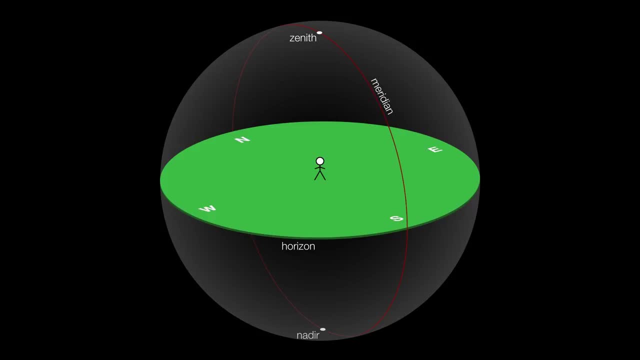 point in the sky from our perspective. So let's just say we have a star and we can describe its position above the horizon. We do that by tracing a line directly to the horizon, that's, directly underneath our star, and drawing an angle up to the star. 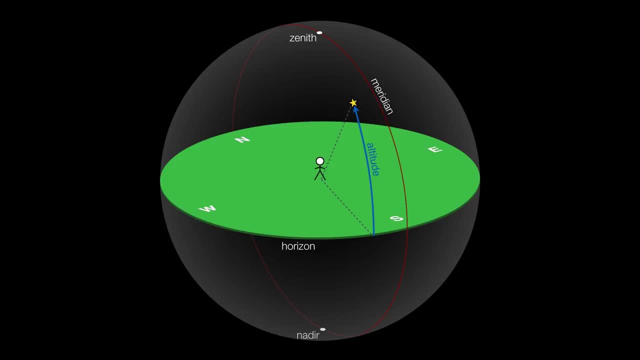 So this is the star's altitude, and we define altitude as zero degrees at the horizon and plus 90 degrees at the zenith. So the zenith is directly overhead. you could just draw a 90 degree angle from the horizon to the zenith. By the way, we can also describe the altitudes of objects below the. 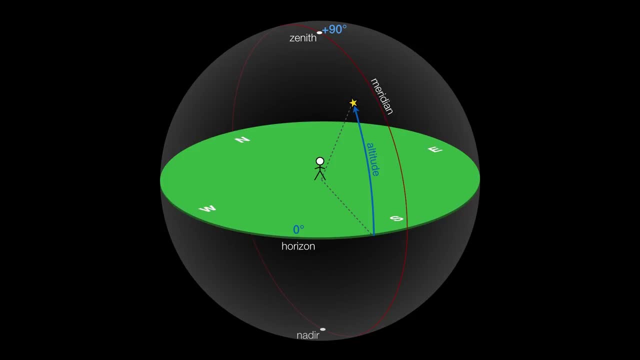 horizon by using negative values. So it's zero degrees at the horizon and minus 90 degrees at the zenith. Now we can also work out where our star is at the horizon, So we can draw a line that's along the horizon. we need to look, and to do that, we start at due north and we just trace a. 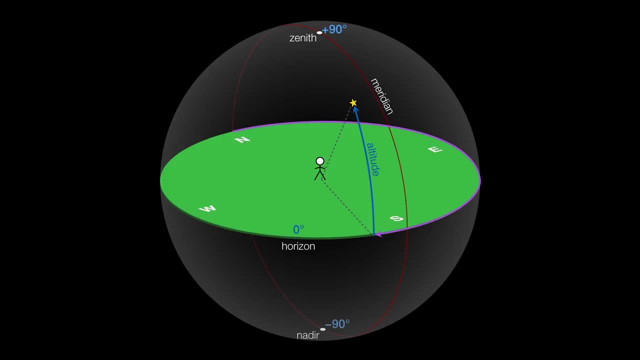 clockwise angle until we arrive directly underneath our star, on the horizon, And this angle is called the star's azimuth. So azimuth begins at zero degrees due north, followed by 90 degrees due east, 180 due south and 270 due west, And for this reason, since it's aligned to the horizon, it's sometimes 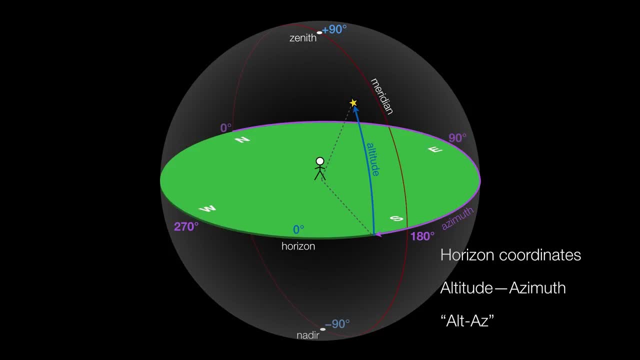 coordinate system, or sometimes alt azimuth or alt az, just for short. Anyway, if you could lie down, it would look like you're looking up into a giant dome and that dome would look a little bit like this. This is what we would see if we had fisheye vision, or even if you could just lie down in a 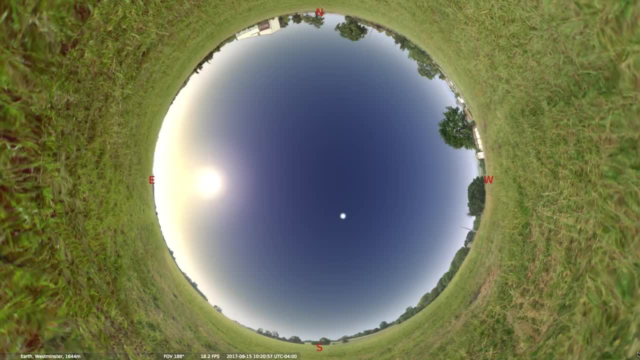 field with your head oriented toward the north and your feet toward the south. If you used your peripheral vision, you could kind of build up an image like this in your brain. You can sense out the horizon. So the horizon is the great circle with the grass drawn on it, and anything that is at the horizon has an 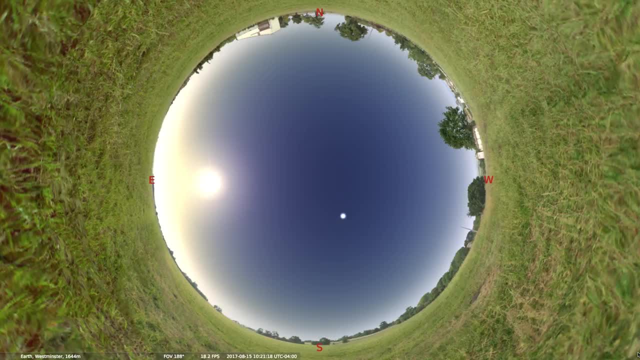 altitude of zero degrees. The point directly overhead is the zenith, which we can represent like this, with the green letter Z, And you can see that this is morning. It's near where I live and you'll see that the Sun is up And because it's the morning, the Sun is somewhere in the eastern half of the sky and it is just above the horizon. 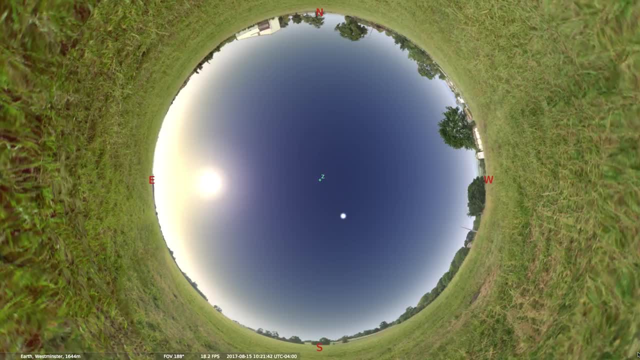 The bright object to the five o'clock position of the zenith, that is, our moon. So the moon is high up, but somewhere in the southwestern sky. So let me go ahead and draw the meridian, this green line arcing from due north, arcing upward through the zenith to due south, And again, this is a little bit tricky but it's worth a try. 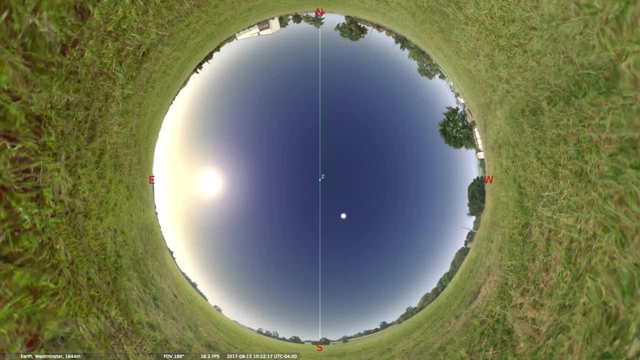 but you just want to remember that you are kind of looking into a dome, So the closer something is to the center of our screen, the higher in the sky or the greater its altitude above the horizon- Okay well, I don't want to have to make you listen to me talk for 24 hours. 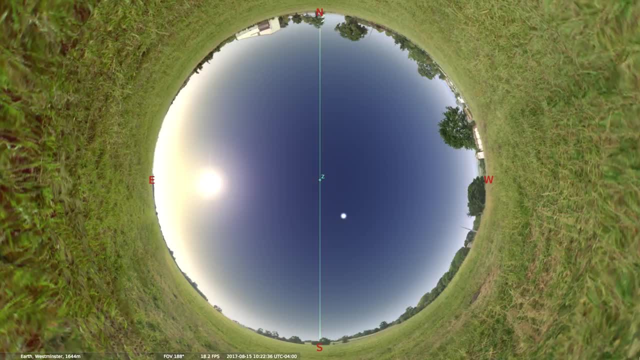 So what I'm going to do is just go ahead and speed up time And we're just going to watch the sun make its way throughout the day today. Okay, so the sun's getting a little bit higher and it's kind of moving in a southeastern direction. 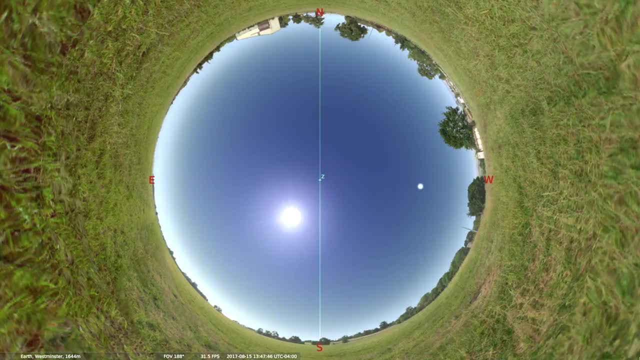 getting closer to the southern horizon And now you'll notice it's about to do what we call transit the meridian. So this point right here, this would represent our local noon. This is not to be confused with 12 o'clock noon.